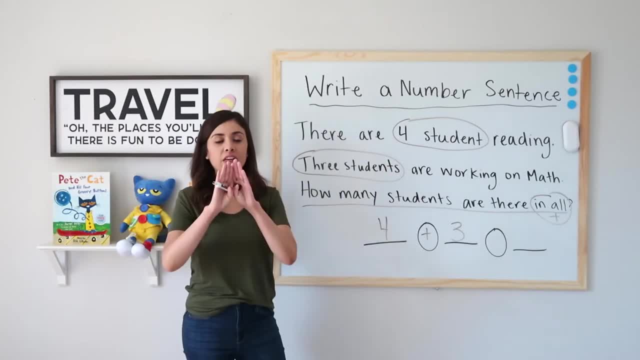 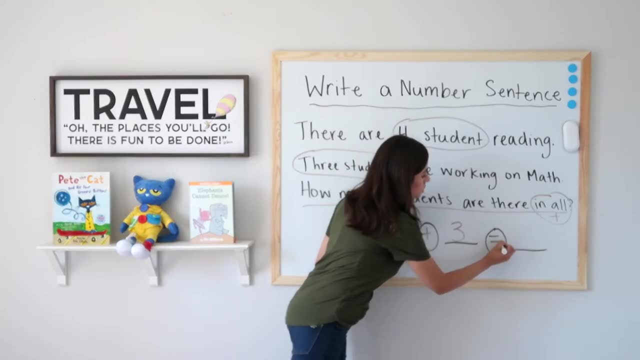 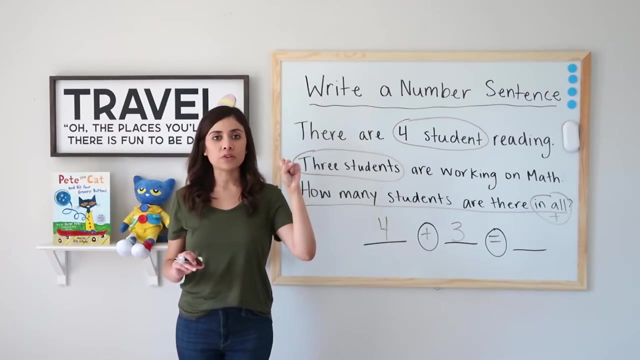 Good, because I want to take part and part and put them together to make the whole. So I have four plus three equals. let's see what four plus three equals. Hold a fist and say four and we're gonna jump up three. 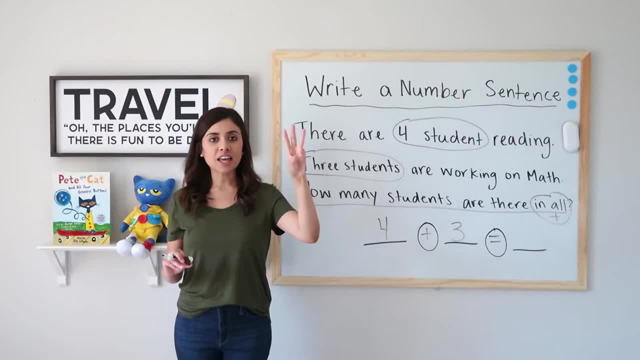 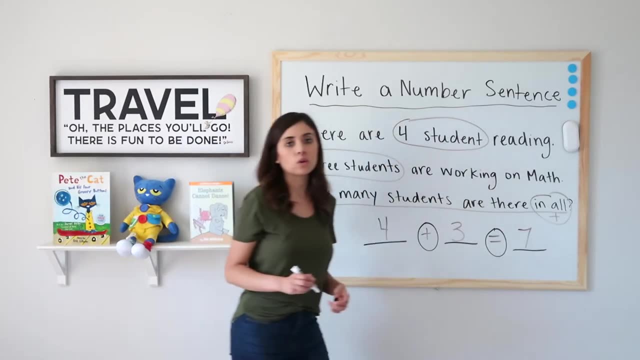 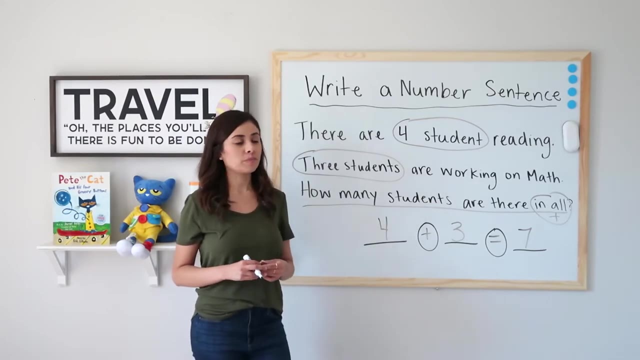 Ready. Four, five, six, seven, Four plus three is seven, Seven is my whole, and it is also called the sum, because sum is the answer to my addition problem. So let's go ahead and take a look at a second example. 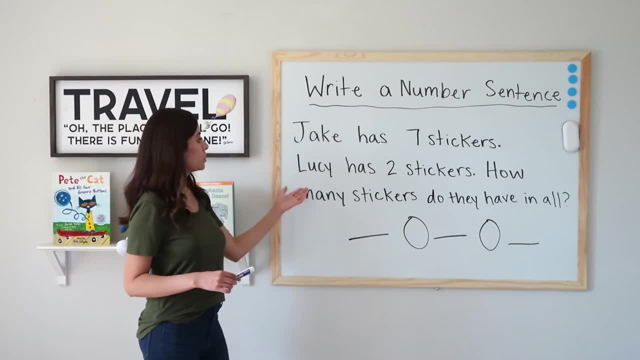 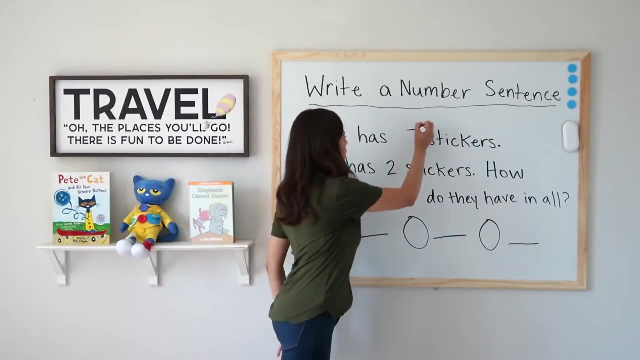 It says: Jake has seven stickers. Lucy has two stickers. How many stickers do they have in all? Remember, the first step is to circle what I already know. I know that Jake has how many stickers? Seven. Good, So I will circle seven stickers. 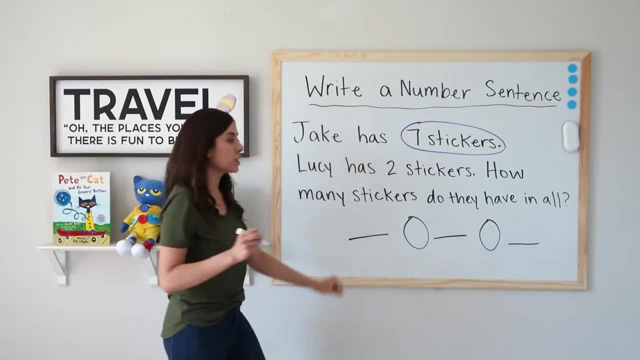 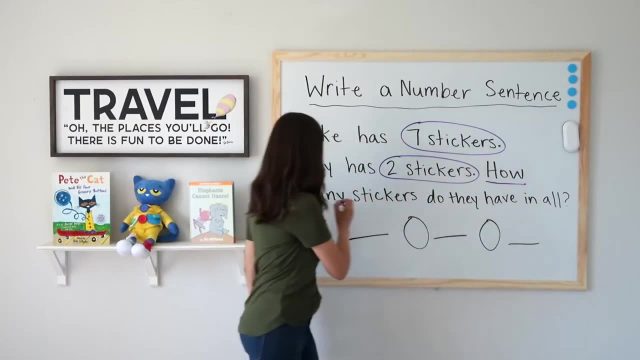 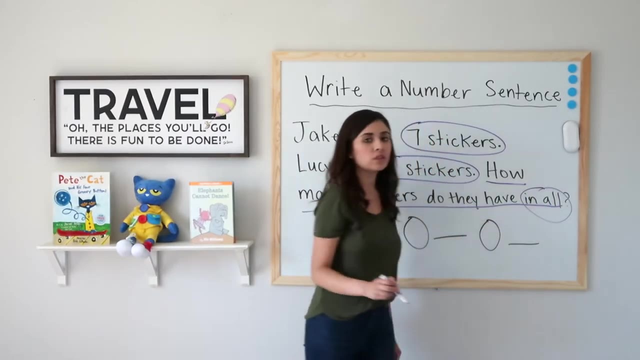 Lucy has. how many stickers? Two Good. So I will circle two stickers and I want to know how many stickers do they have in all And in all means to add Very good, So I will take my two parts, seven and two. 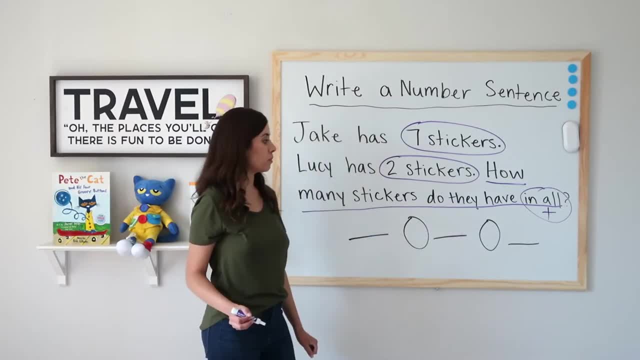 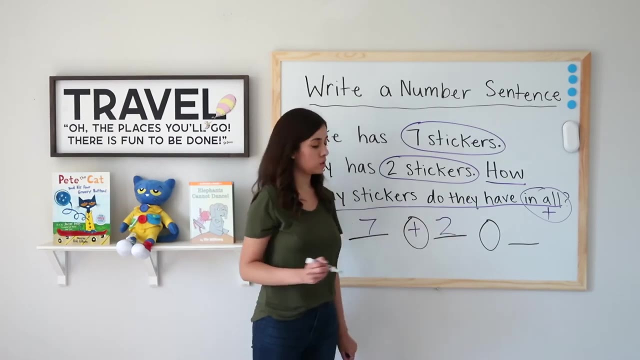 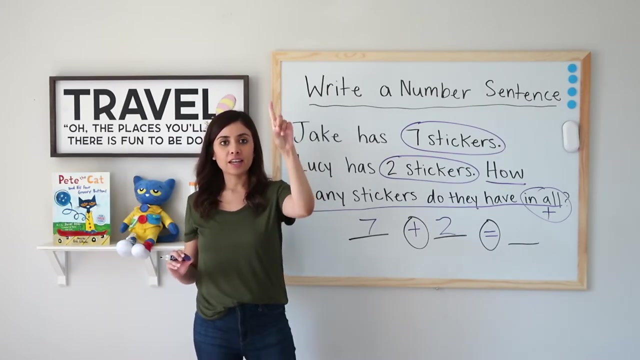 Very good- 2 and write them down in my number sentence: 7 and 2.. And I know that I have to add them: 7 plus 2 equals right, So I have 7 and I jump up 2.. 7,, 8,, 9.. 7 plus 2 is 9.. 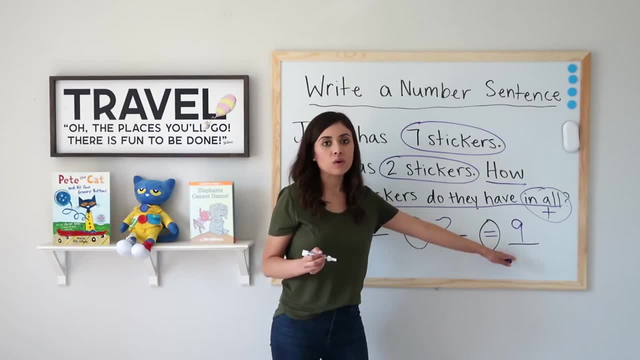 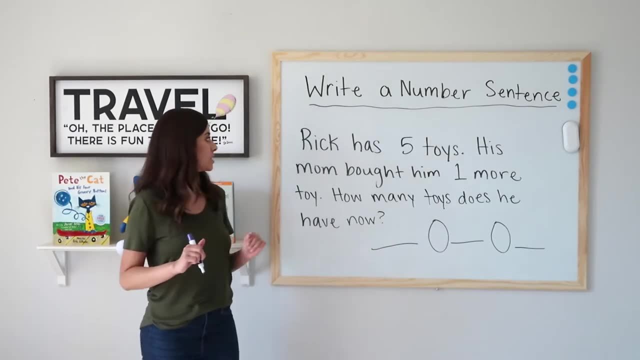 9 is my whole, and it is also called the sum. Okay, so on to the next example. It says Rick has 5 toys. His mom bought him one more toy. How many toys does he have now? So first, before we look into anything else, let's circle what we already know. 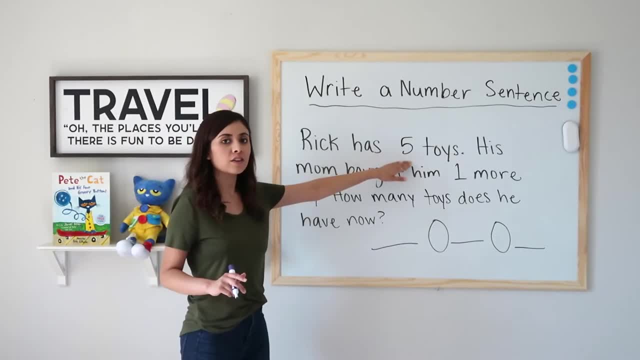 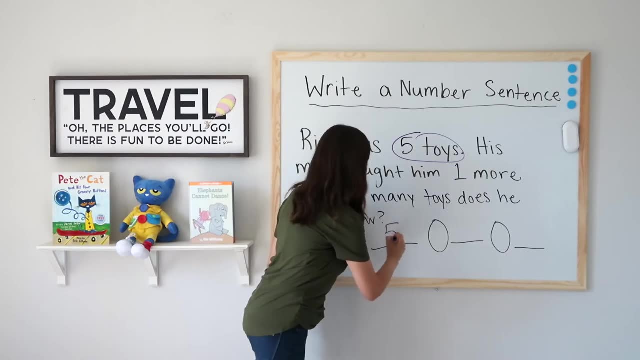 I know that Rick started off with how many toys? 5.. Good, You know what. I'm actually going to go ahead and write that part down already. 5.. His mom bought him one more toy. How many? One more. 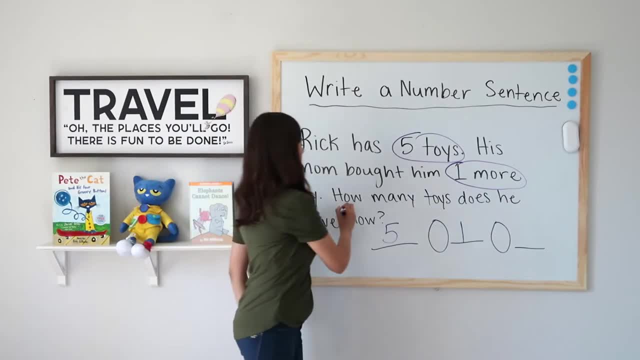 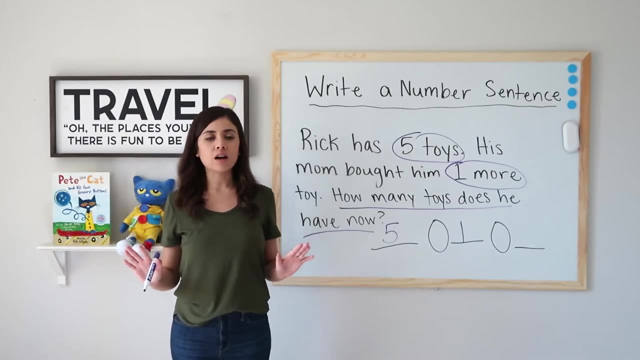 Okay, so I want to know how many toys does he have now? And if you notice, my question does not have the words in all. We know that in all means to add, But how do I know what to do here? So this is where I have to really think about real world problems, okay. 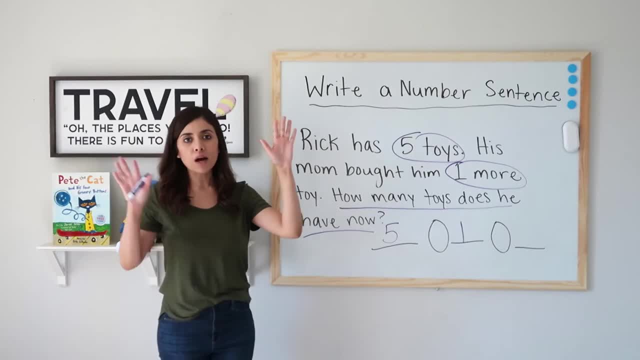 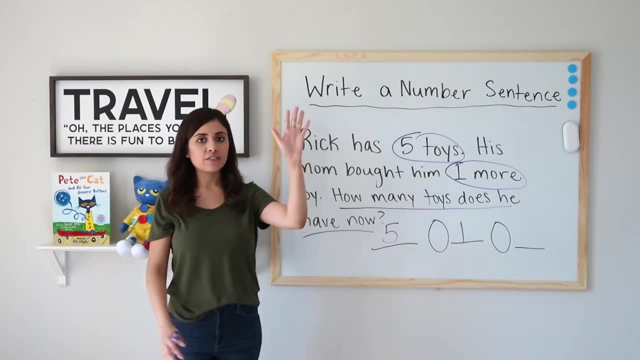 I have 5 toys and I bought another one. Am I adding that toy or subtracting it? If I have 5 and we get from the store one more, do I add that one to the 5? Or did I take away from the 5?? I added, Very good. 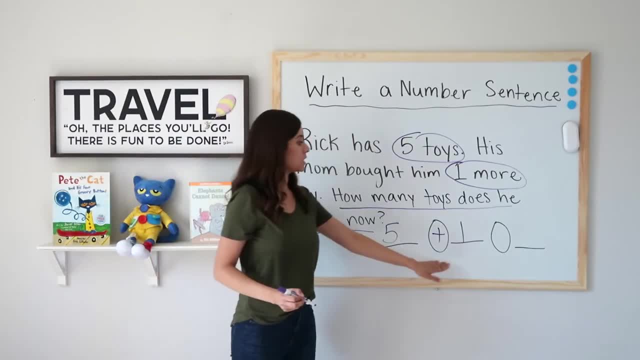 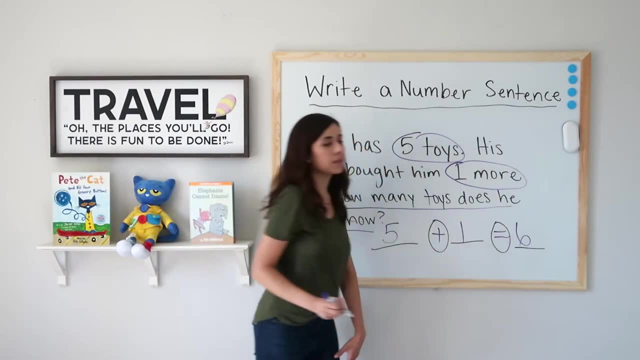 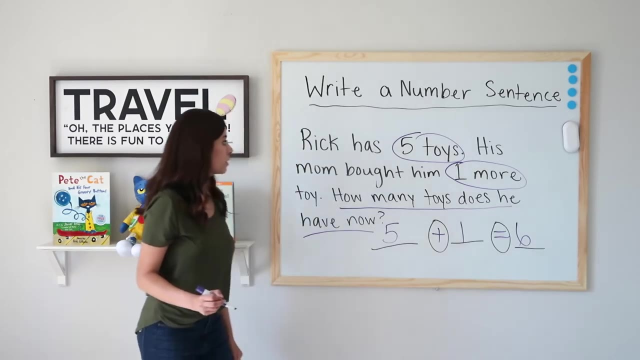 I started with 5 plus one more equals 6.. Good, Because I have 5, I jump up 1 and that's 6.. 5, 6.. Very good Now if the problem were to say: his mom took one over. 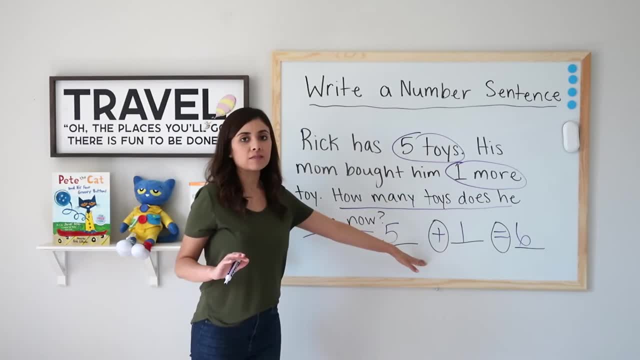 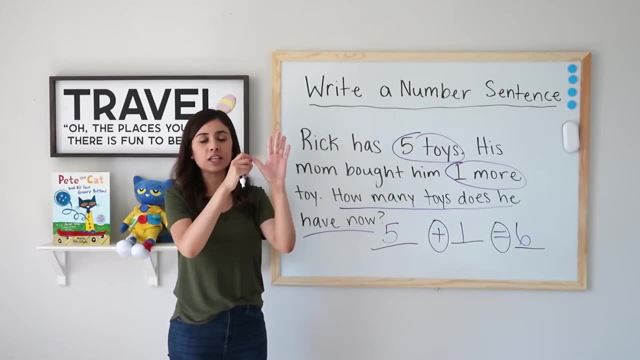 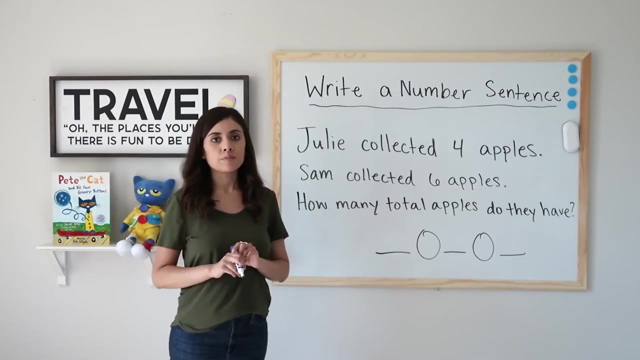 then I would know that I have to subtract because he had 5 and we took one away. Okay, that is subtraction, But here he had 5 and one was added from the store, right, Very good. This problem says: Julie collected 4 apples, Sam collected 6 apples. 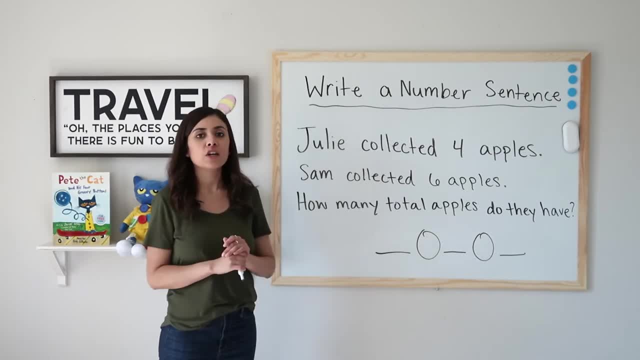 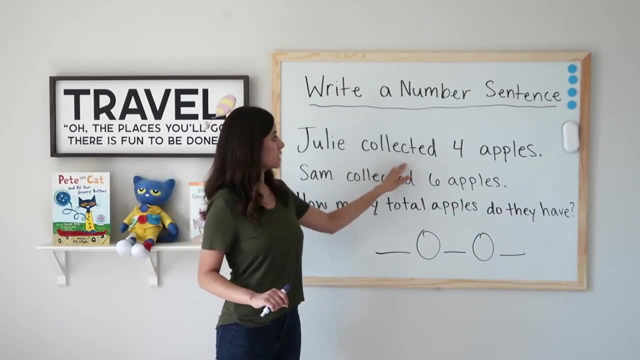 How many total apples do they have? Remember? the first thing we have to do is add. Remember. the first thing we want to do is circle what we already know. So I know that Julie collected how many apples? 4. Good, 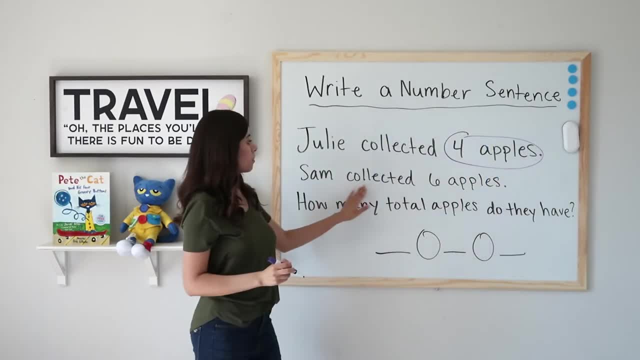 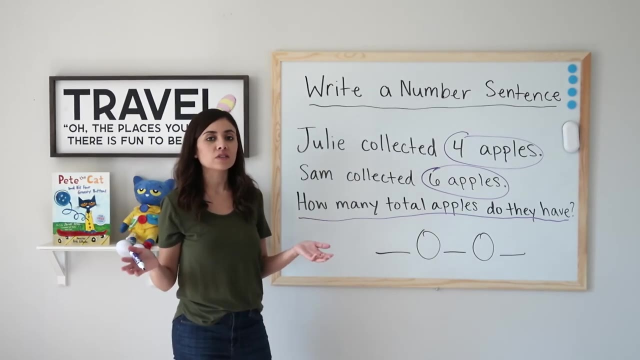 Let's circle 4 apples. Sam collected how many? 6.. Very good, I want to know how many total apples do they have? Again, I don't see the words in all. Let's go back and look at our question.